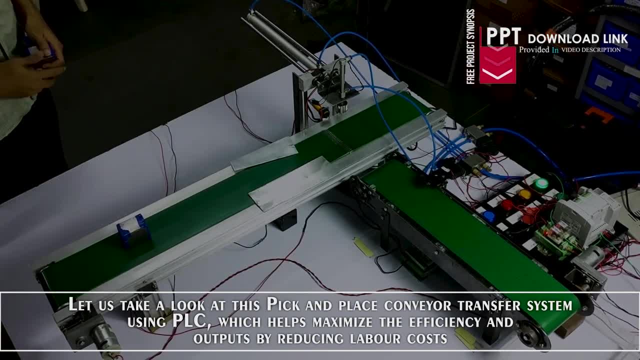 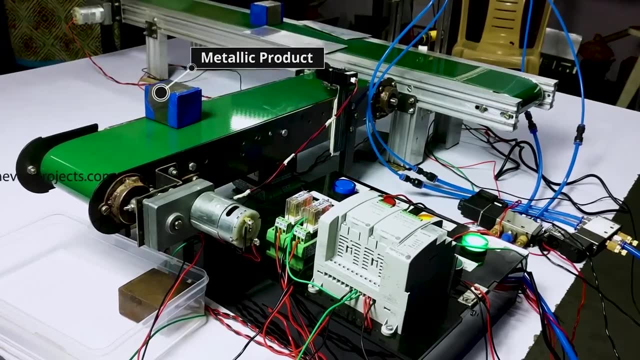 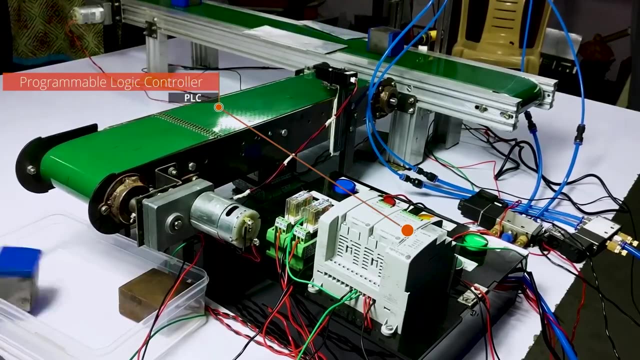 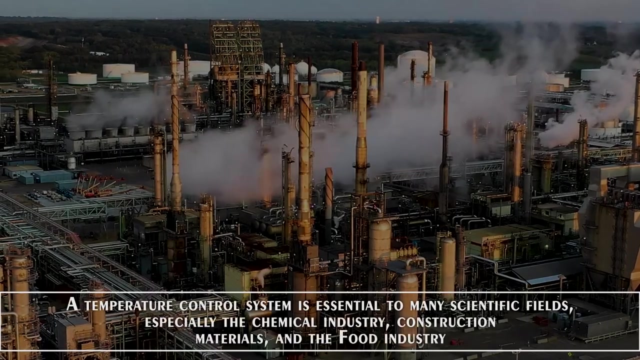 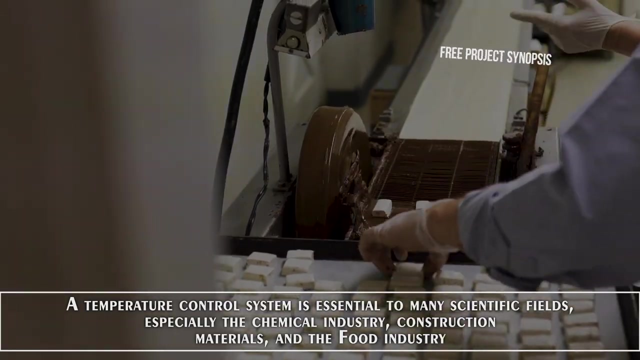 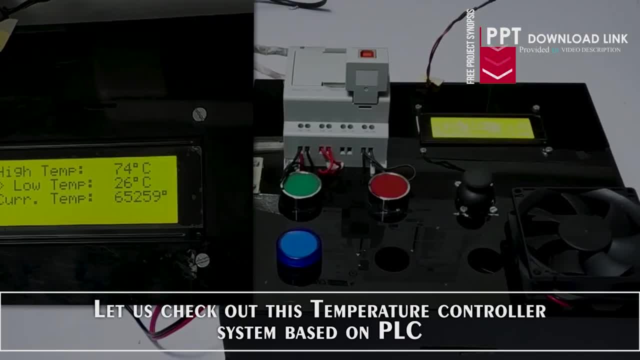 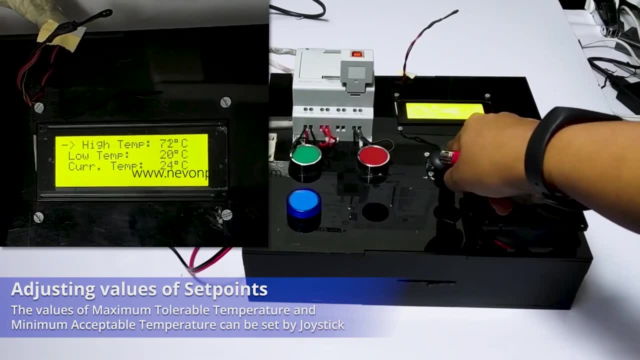 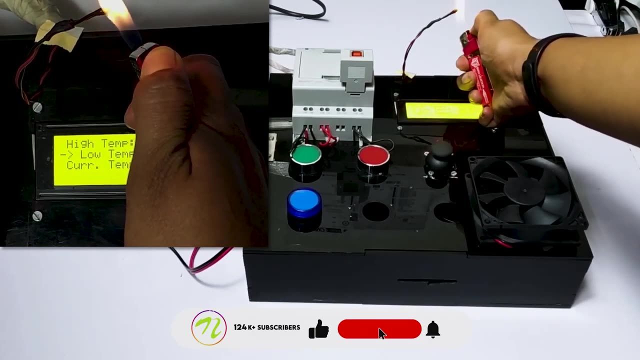 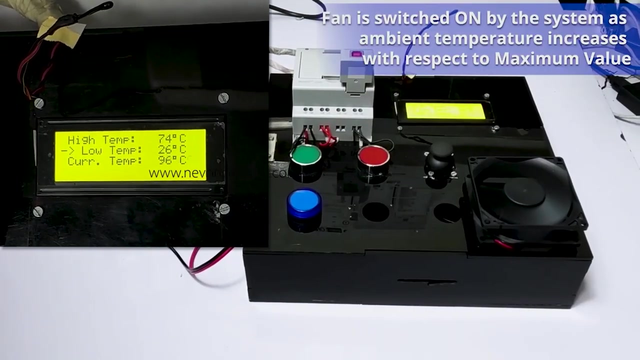 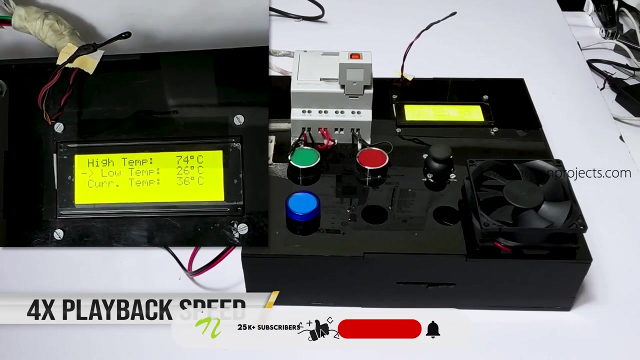 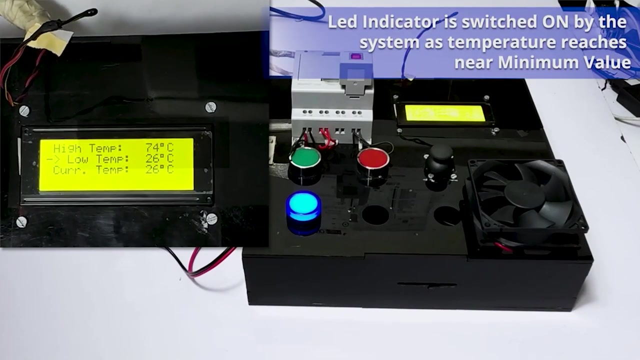 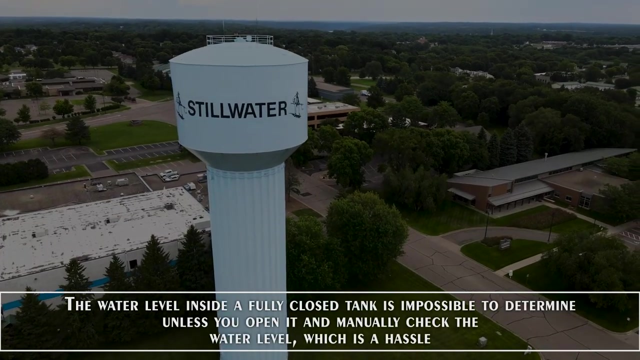 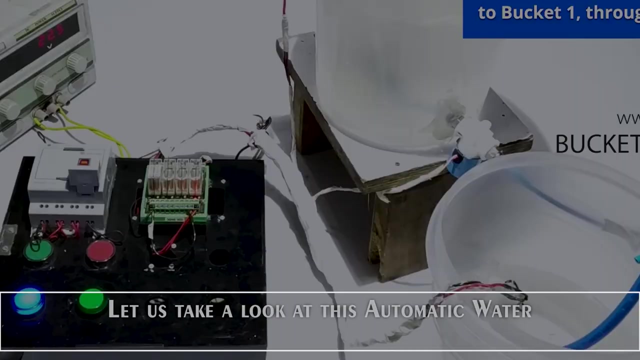 Let us check out this temperature controller system based on PLC. Temperature controller system based on PLC. Temperature controller system based on PLC. Automatic Water Level Control System. using PLC. The water level inside a fully closed tank is impossible to determine unless you open it and manually check the water level, which is a hassle. 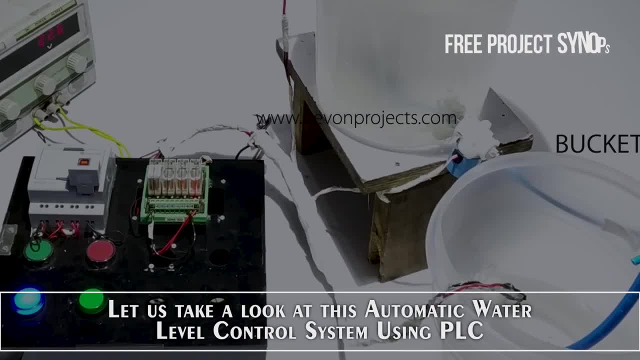 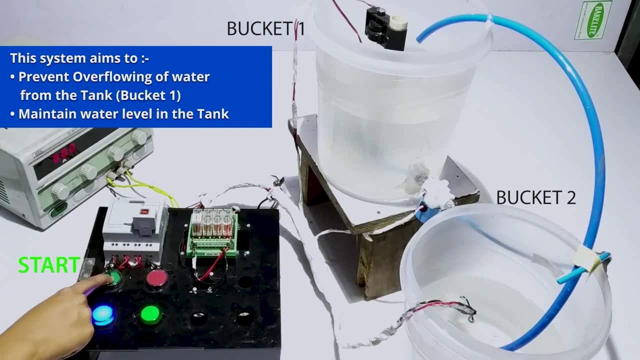 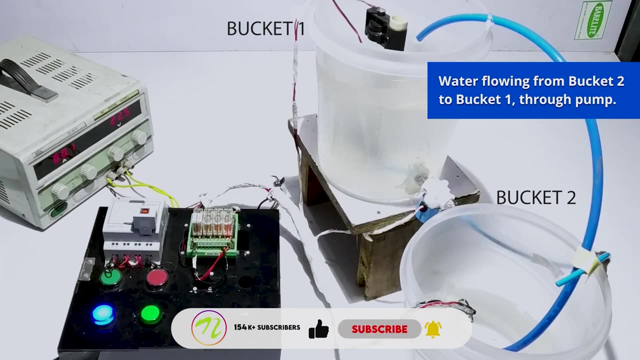 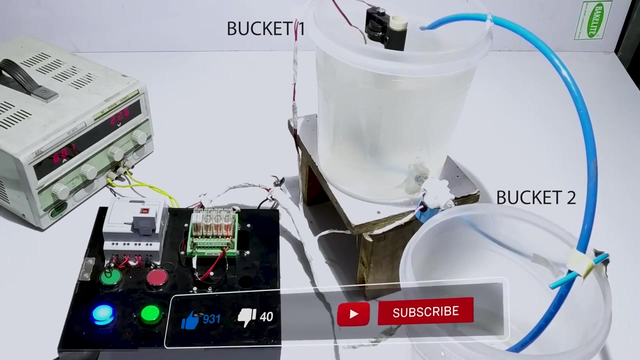 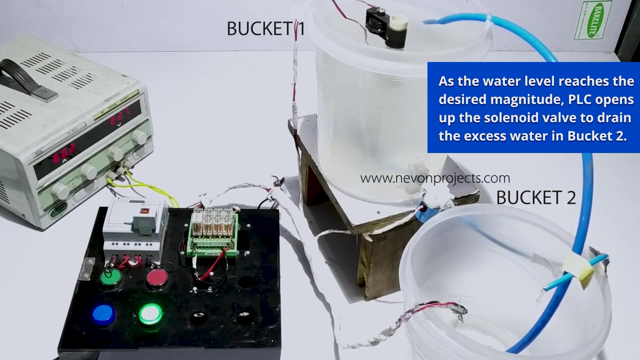 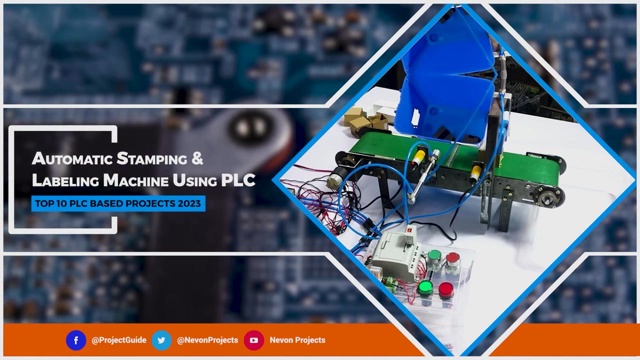 Let us take a look at this automatic water level control system using PLC. This system helps prevent overflowing water from the tank and helps maintain the water level. Automatic Stamping and Labeling Machine using PLC. All product automation processes require labeling or stamping as the last step to brand the 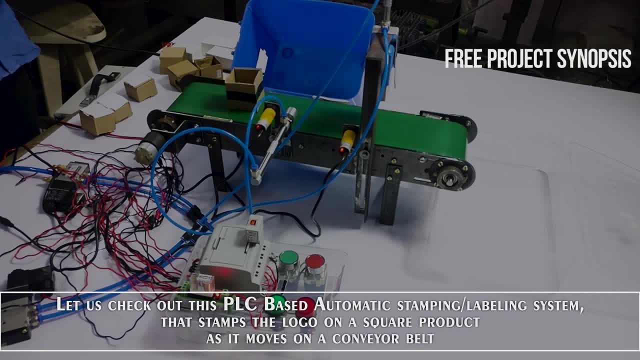 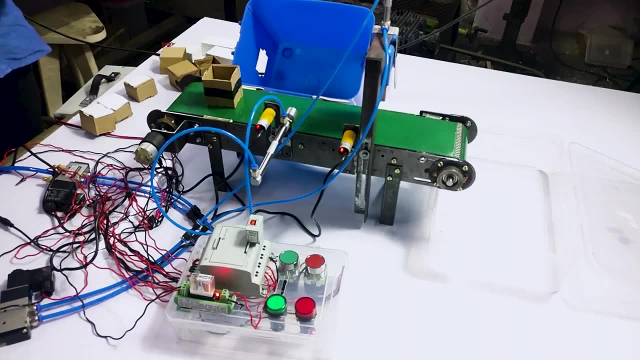 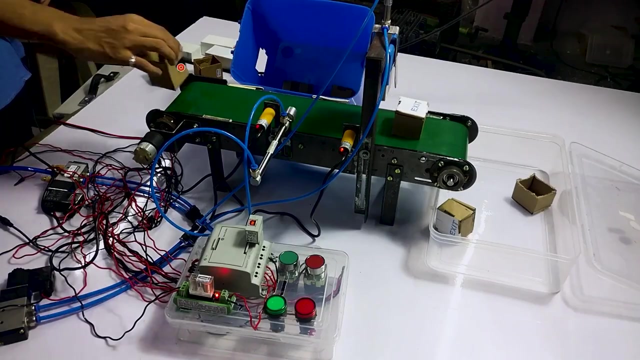 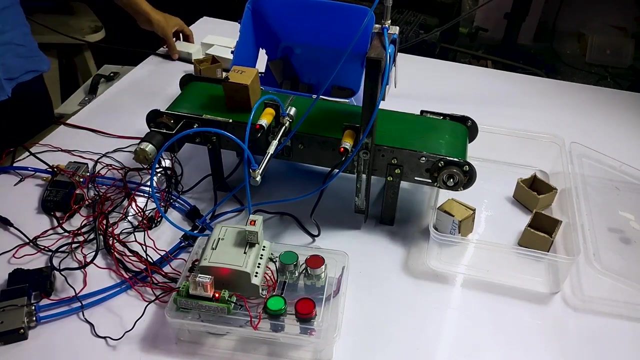 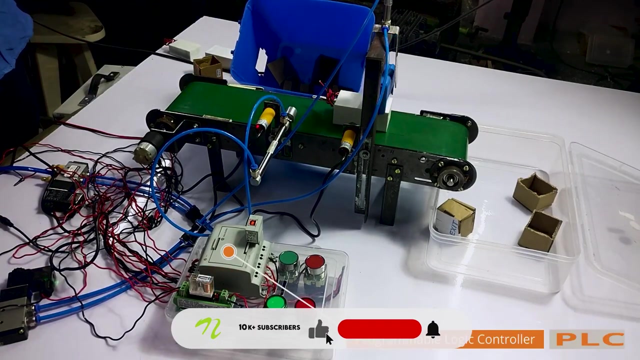 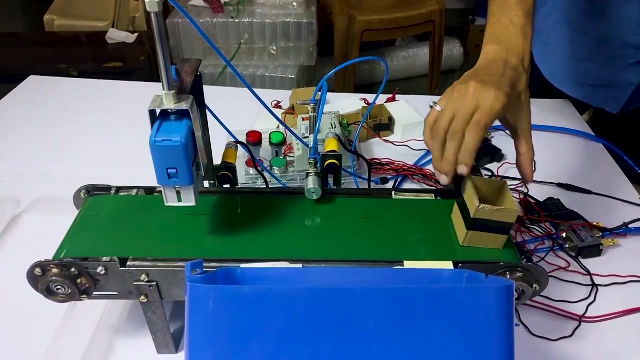 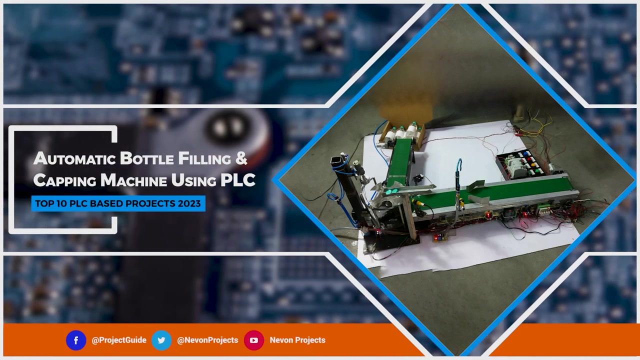 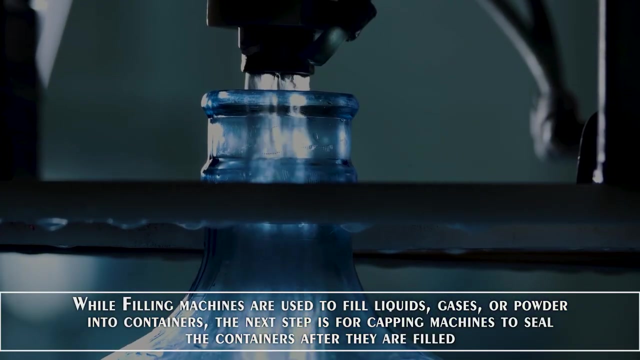 finished product. Let us check out this PLC-based automatic stamping and labeling system that stamps the logo on a square product as it moves on a conveyor belt. Automatic Bottle Filling and Capping Machine using PLC. While filling machines are used to fill liquids, gases or powder into containers, the next: 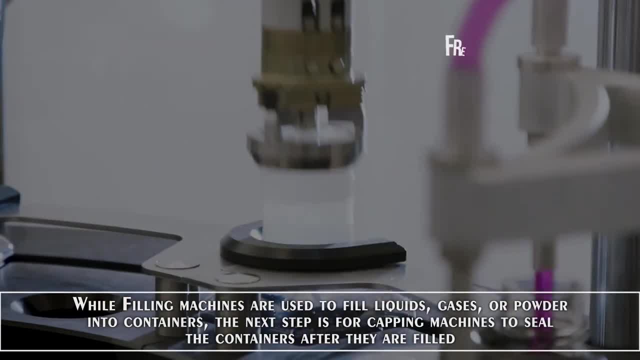 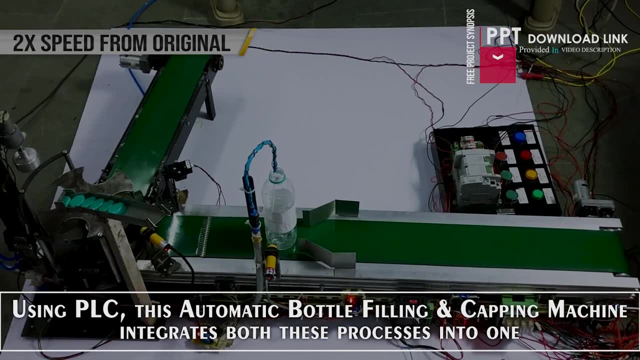 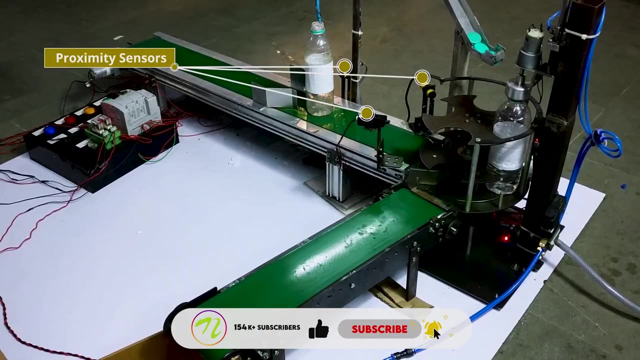 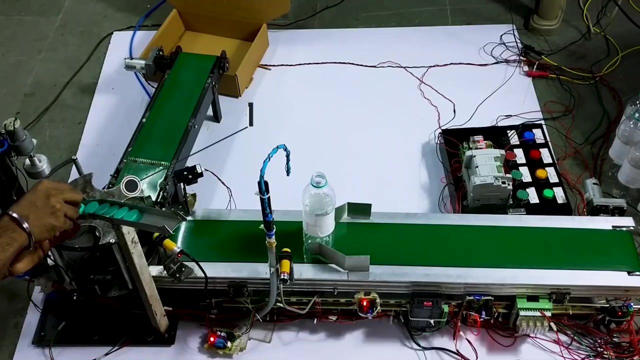 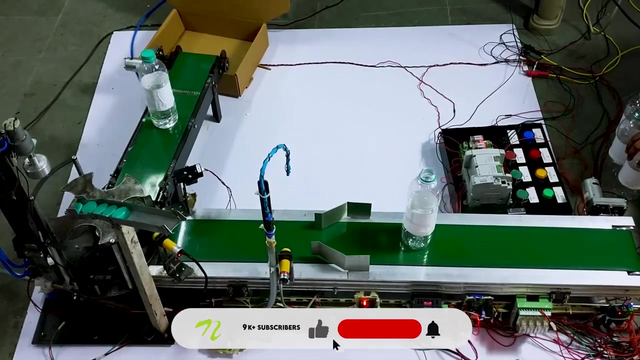 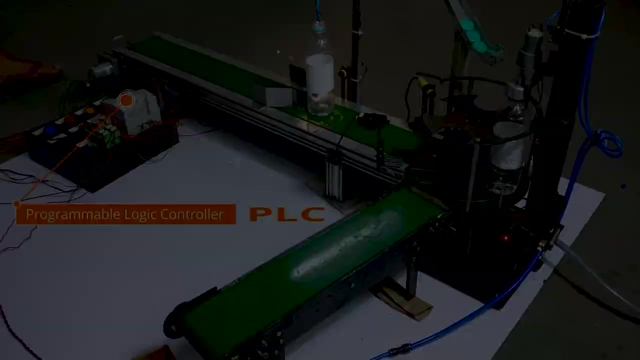 step is for capping machines to seal the containers after they are filled Using PLC. this automatic bottle filling machine can be used to seal the containers after they are filled. Automatic Bottle Filling and Capping Machine integrates both these processes into one PLC-based Paper Cutting Machine. 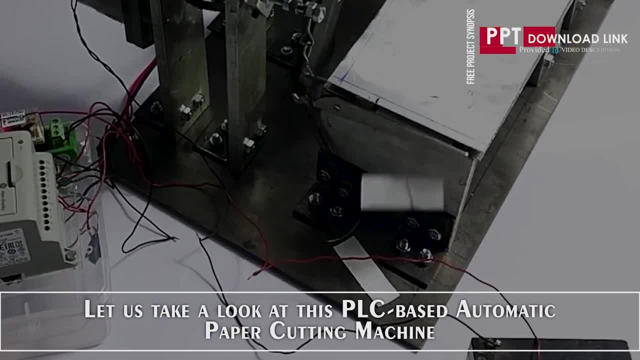 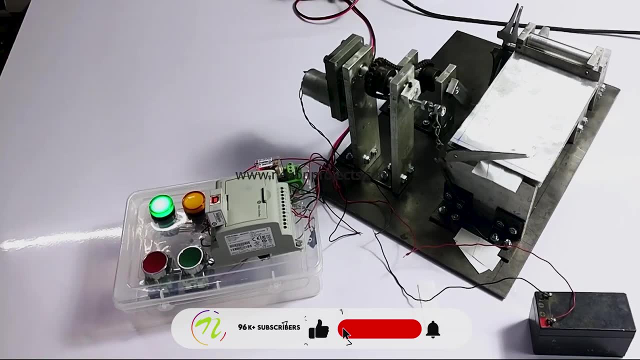 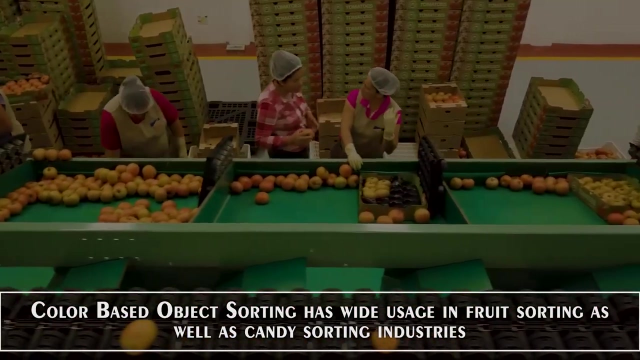 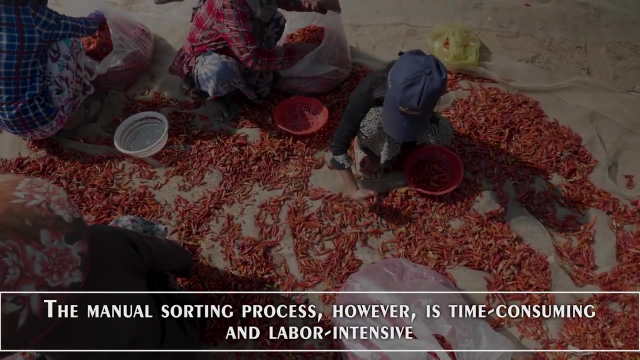 Let us take a look at this PLC-based automatic paper cutting machine. long Color Product Sorting Using a Pneumatic Conveyor Belt. Color based object sorting has wide usage in fruit sorting as well as candy sorting industries. The manual sorting process, however, is time consuming and labor intensive.